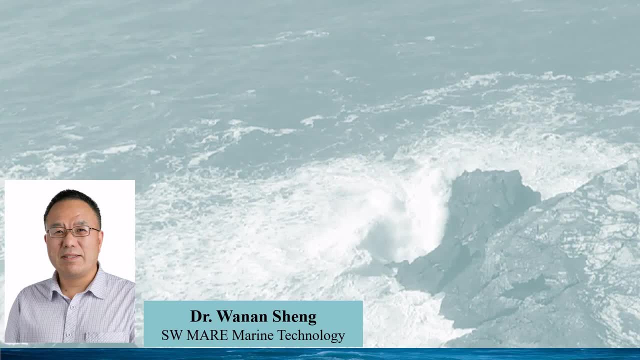 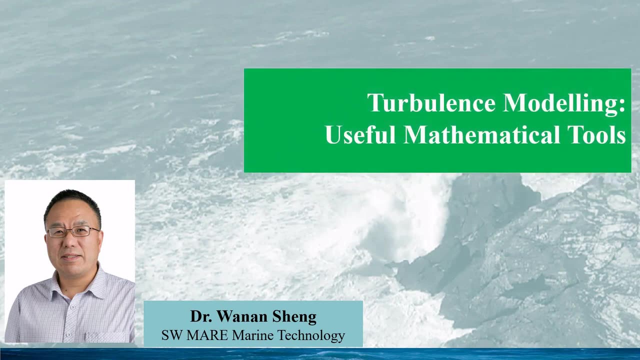 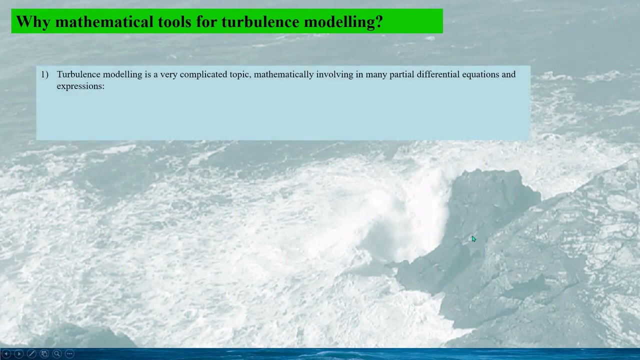 Hello, welcome to my talk all about fluids. This talk is on the mathematical tools for turbulence modeling. I mean to provide the useful tools as well as some tricks in the mathematics of the turbulence modeling. Turbulence modeling is a very complicated topic mathematically. 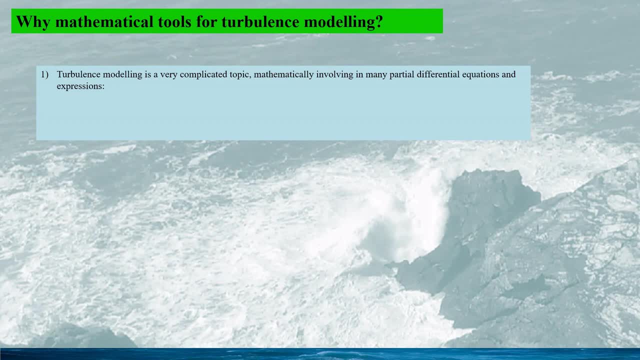 involving many partial differential equations and expressions: Navier-Stokes equation, Reynolds averaged Navier-Stokes equation, Reynolds stress tensor, turbulent transport equation, and etc. The conventional mathematical formulas for this partial differential equation would be very complicated and difficult to understand in many cases, if all the 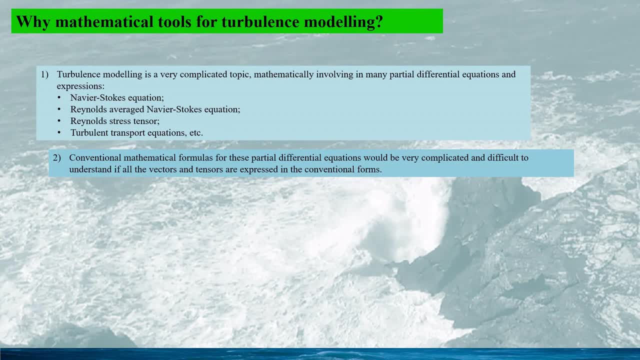 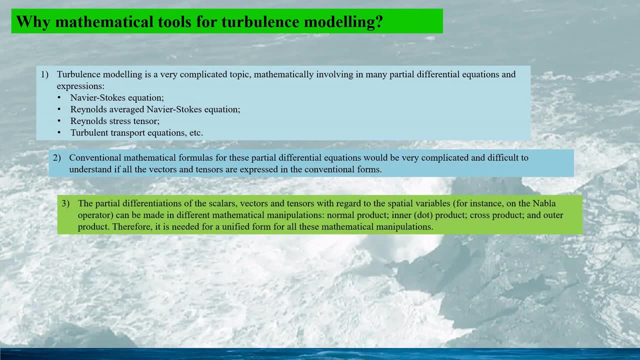 vectors and the tensors are expressed in the conventional form. The partial differentiations of the physical parameters, including scalars, vectors and tensors, with regard to the turbulence modeling are very complicated. In addition to the special variables, for instance on the Nabla operator, can be 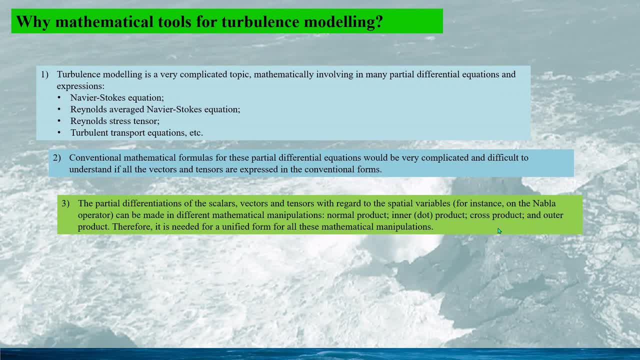 made in different mathematical manipulations: normal product, inner product, cross product and outer product. therefore, it is needed for a unified form for all these mathematic manipulations. A solution to the above problem is the Einstein summation convention or Einstein notation. 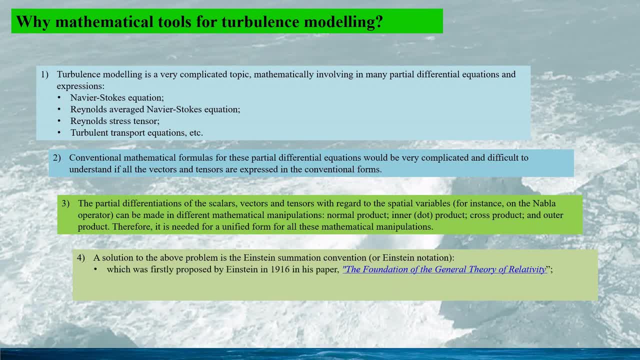 Einstein's summation convention was first proposed by Einstein in 1916 in his paper. the foundation of the general theory of relativity and ever since the notation has been widely accepted and applied in physics includes fluid dynamics. Most of the turbulence models have been written in Einstein notation because it gives the 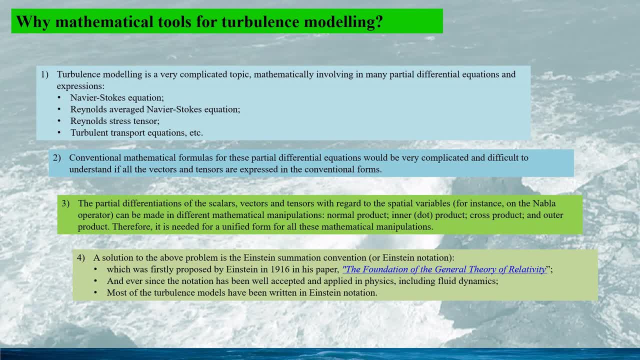 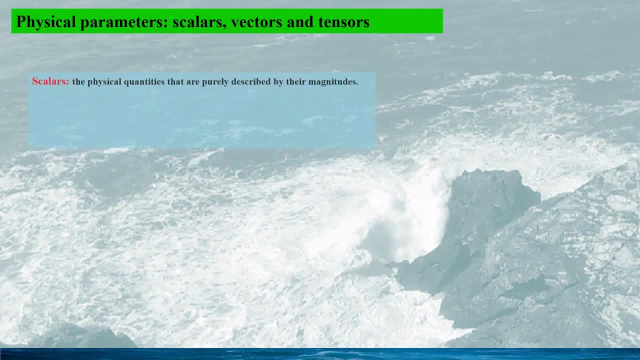 simplest mathematical expression for the turbulent transport equations. There are different physical parameter types for representing the different physical parameters. for instance, the scalars, which might be the simplest parameters we are using daily, are the physical parameters that are purely described by their magnitudes. This includes 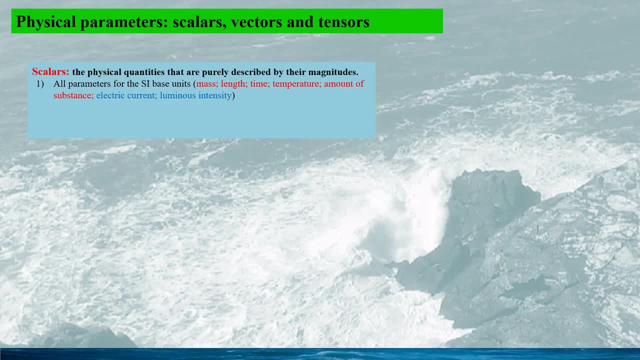 the physical parameters for the SI base units: mass length, time temperature and time temperature, amount of substance, electric current, luminous intensity. The first five of the base units may be used in fluid dynamics. All other units are derived from these seven base units called derived. 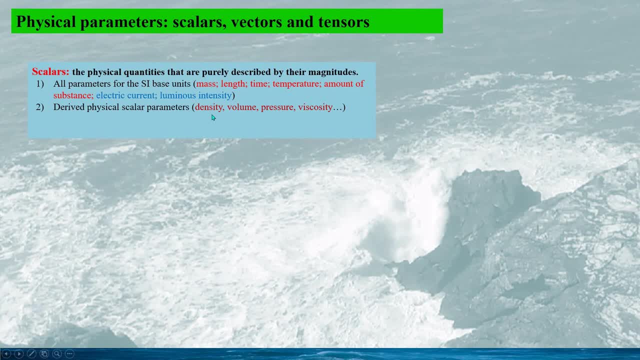 physical parameters, for instance density, volume, pressure, viscosity, etc. There are also other derived groups of scholars named the non-dimensional parameters, including the famous Reynolds number, Mach number, fluid number, etc. Mathematically, scholars have a dimension of 1x1,. 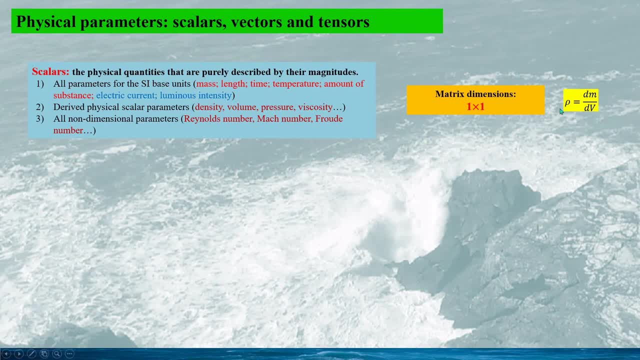 that is 1x1 matrix. for instance, the fluid density is a such scalar, defined as the mass derivation. with regard to volume Vector, are the physical parameters which are described with both magnitude and direction, including force, moment, momentum, displacement velocity. 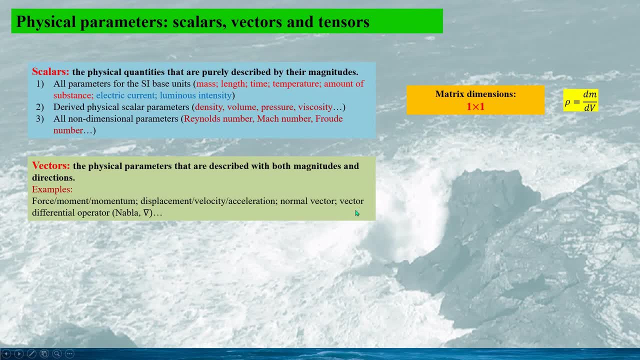 acceleration, normal vector, vector, differential operator, that is, Nabla, etc. mathematically a vector has a dimension of 3 times 1, so the vector velocity can be written in these 3 times 1 matrix here u, v and z. 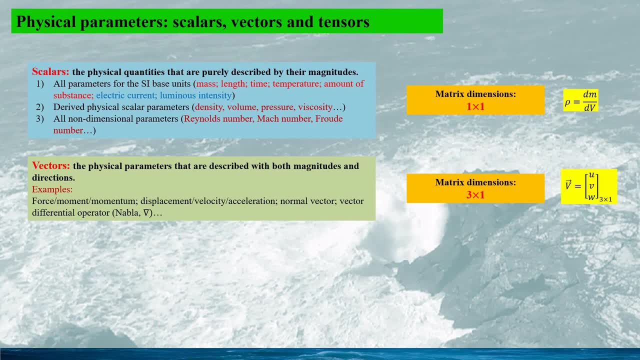 and w are the velocity components along x, y and z-axis respectively. In real world we can understand vectors easily. for instance, when we move our weight. we know how to apply the force, the magnitude and the direction of the applied force, so we can move the weight. 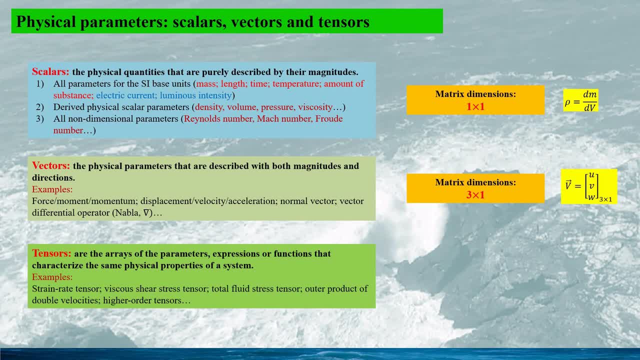 Tensors are the array of the parameters, expressions or functions that characterize the same physical properties of a system, for example strain rate tensor, viscous shear stress tensor, total fluid stress tensor, outer product of double velocity and higher-order tensors. Mathematically, a second-order tensor has a dimension of 3 times. 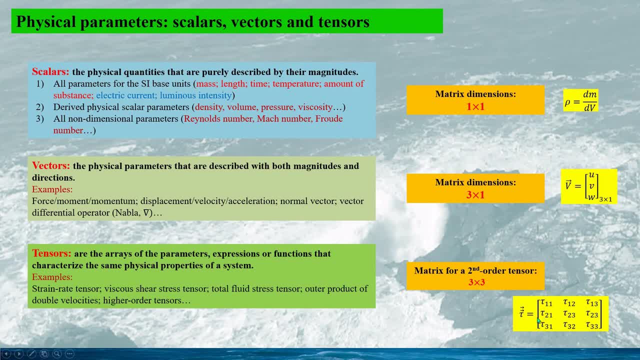 3,. for example, the shear stress tensor tau double arrow is given by a matrix of 3 times 3,. for example, the shear stress tensor tau double arrow is given by a matrix of 3 times 3,. 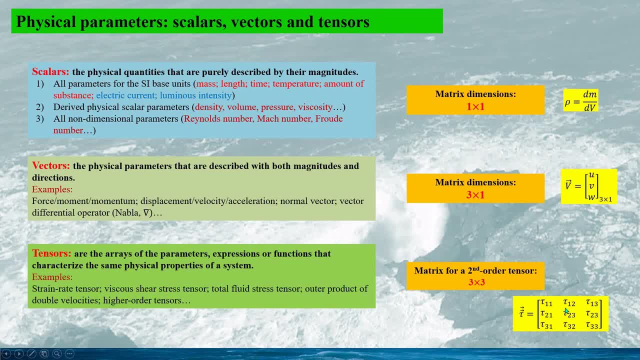 for example, the shear stress tensor tau double arrow is given by a matrix of 3 times 3,. here the components have specific meaning. for instance, tau-1,2 means the tensor acts in the x-direction, which is indicated by the first index. 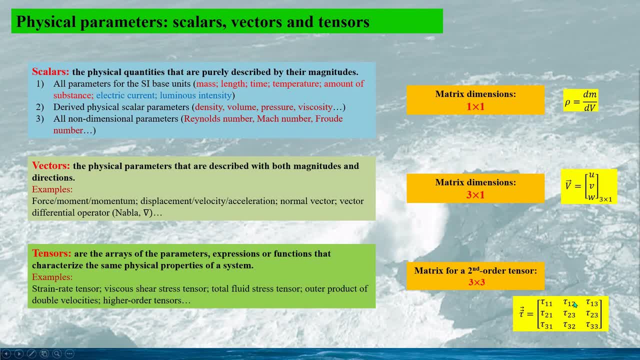 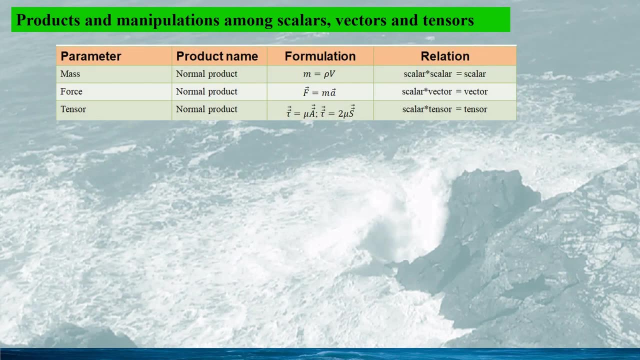 1 here upon a surface of a constant y. the second index, 2, indicates this Here. in this slide the relation and the manipulations are given for the scalar vector and the tensors. here mass is the scalar defined as the scalar times scalar. 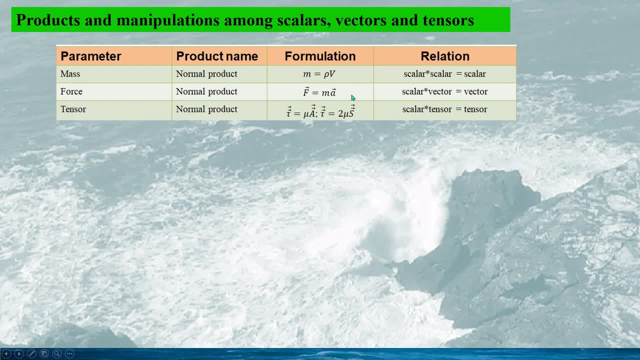 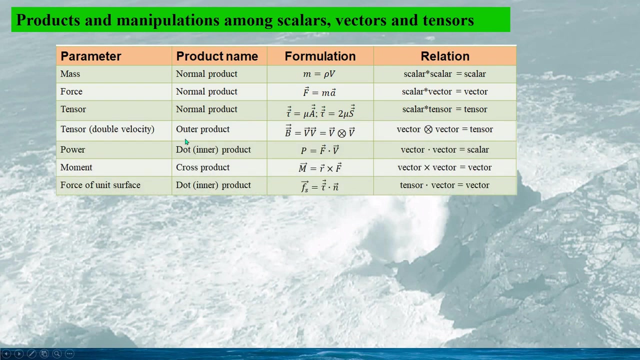 density and the volume force is the vector defined by a scalar m times a vector. acceleration tensor here is given by a scalar time tensor. we have also a tensor due to the outer product of the double velocity given by this. so the dielectric sign means an. 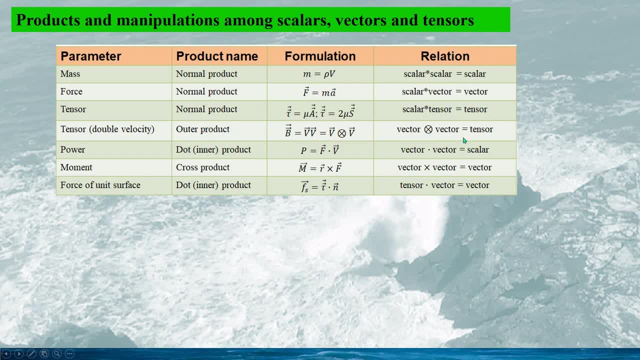 outer product and the power is the scalar given by a vector force: dot times the vector velocity. the moment is given by a cross product of the double velocity and the momentum is given by a cross product of the double velocity, displacement r and the force. 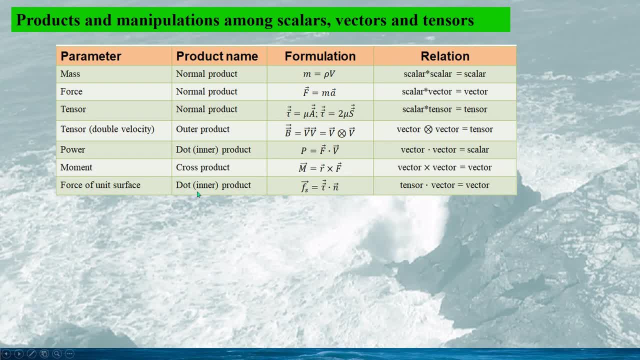 and the force of a unit surface is a dot product or inner product of a tensor and a normal vector given in this form, and we have some mathematical values such as the double dot product, and we have some mathematical values such as the double dot product. 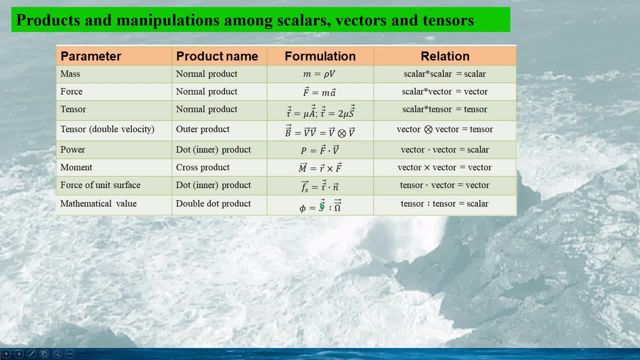 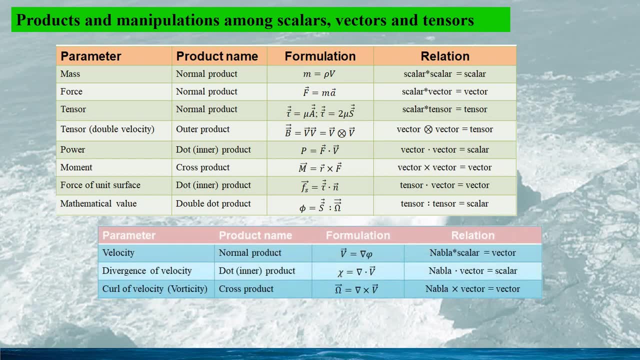 for two tensors given by this. here, Phi is the scalar. We have also a very special vector, differential operator, NABLA, which is a very useful operator in the fluid dynamics and the turbulence modeling, for instance the spatial gradient of a scalar function as this. 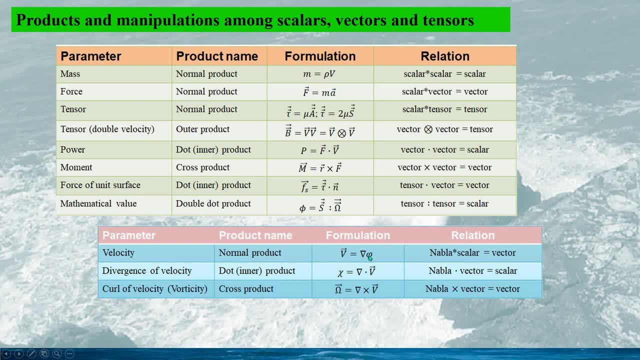 the normal product of NABLA and the scalar function is a vector and the divergence of the velocity is given by NABLA dot, the velocity vector. for an incompressible flow, the divergence of the velocity would be zero and the core of the velocity given by this NABLA dot, the velocity vector. 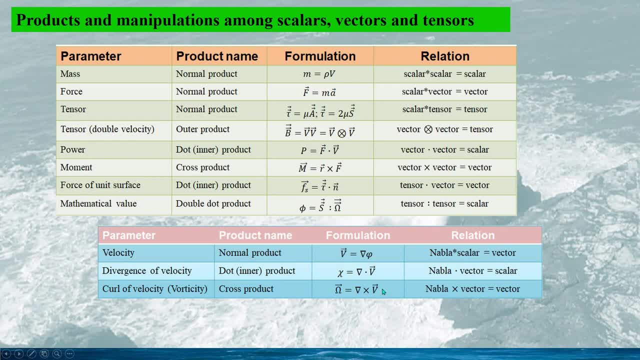 by this labrador cross-timing the velocity vector, we can also have the force of unit volume is a dot product of labrador and their tensor. so we may have the mathematical tensor, the outer product given by labrador, outer times the velocity. 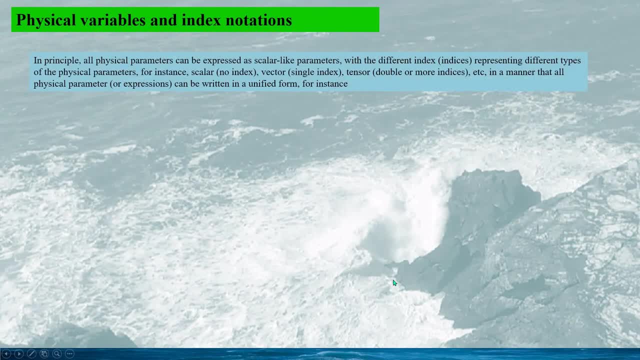 in principle, all physical parameters can be expressed as scalar-like parameters with the different indexes or indices representing the different type of the physical parameters. for instance, scalar is given with outer index and vector is given with a single index and tensor with double or more. 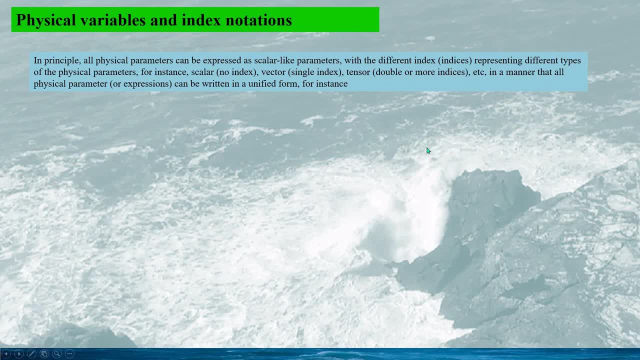 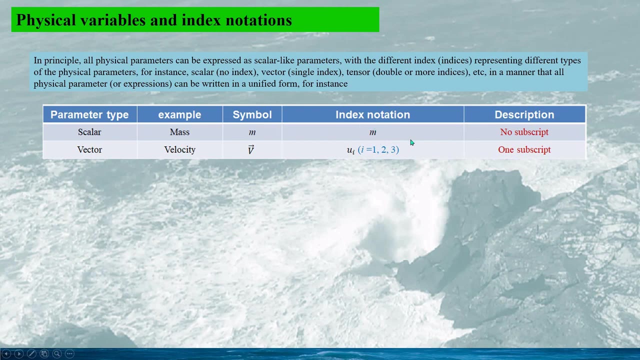 indices, so in such a way that all physical parameters or expressions can be written in a unified form. for instance, the scalar given by this, just simple, with no subscript, and the vector. the velocity is given by a symbol with an index. i here i equals to 1,, 2 and 3,. 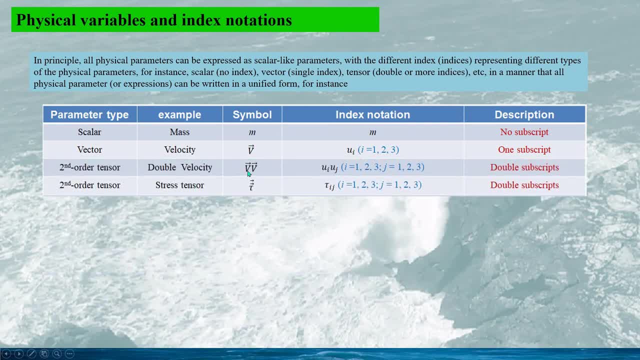 so we have the second-order tensor, for instance the double velocity. so we have this ui and uj here, i equals to 1,, 2 and 3, and this same for j equals to 1,, 2 and 3, and the stress tensor TAU-RR. 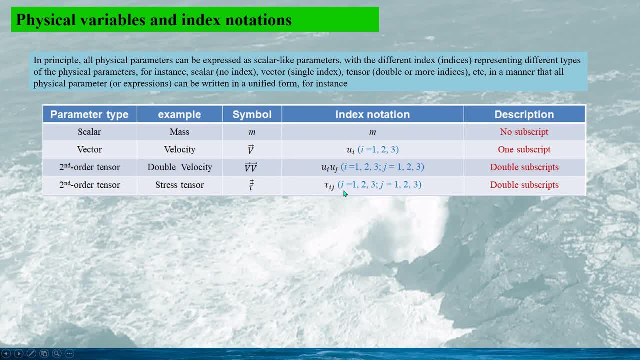 given by TAU-ij. so the second tensor is with double subscript. in the turbulence modeling we may make some higher-order tensor, for instance the triple velocities given by this in vector form, and if we use the index notation we have ui, uj and uk here i j and k equal to 1,, 2 and 3,. 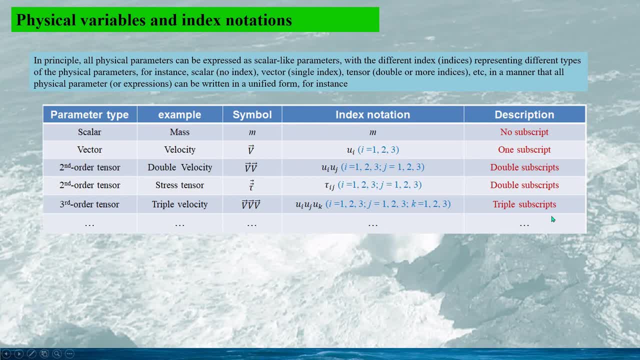 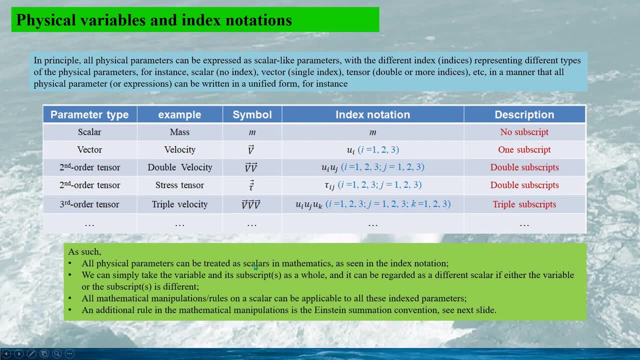 so the third-order tensor is with three subscripts: i, j, k here. so as such, all physical parameters can be treated as scalars and we can simply take the variables and its subscript as a whole and it can be regarded as a different scalar if either the variable or the subscript is. 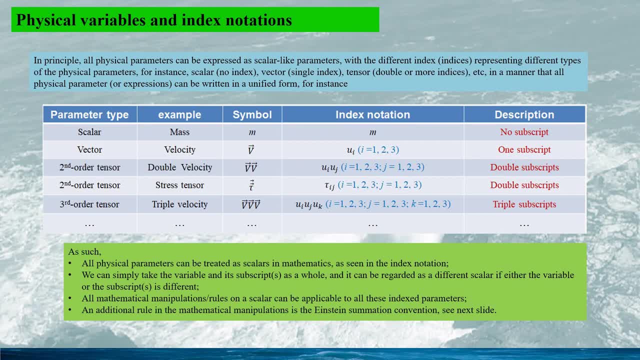 different and all mathematical manipulations and the rules on the scalar can be applicable to all these in-text parameters. an additional rule in the mathematical manipulation for all these in-text parameters is the Einstein summation convention. we will see this in the next slide. 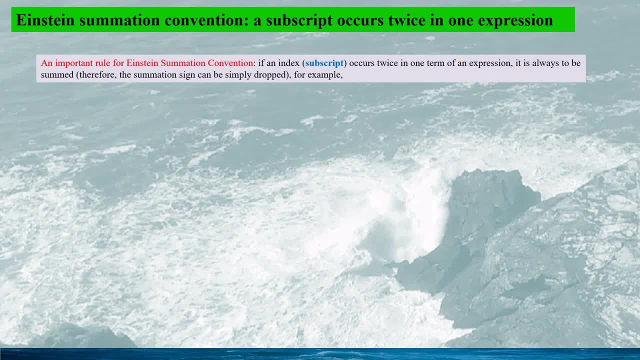 The important rule is the Einstein summation convention. if an index or a subscript occurs twice in a term or expression, it is always summed. therefore the summation sign can be simply dropped. for example, the specific kinetic energy, the energy per unit mass, is given by this. so in: 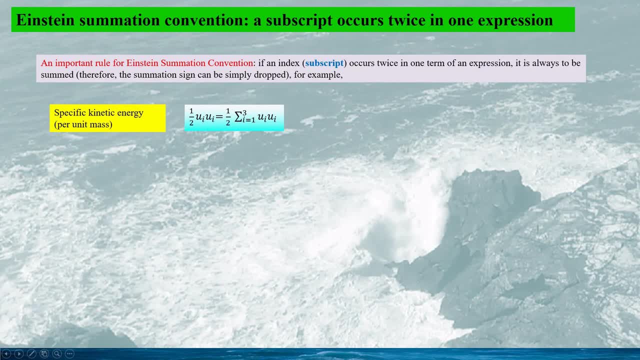 this term index i occurs twice. it means it is a summation as this, but in Einstein's notation the sign for summation, Sigma, is simply dropped. so it is equivalent to this and this. so the result is the scalar, The continuity equation for the incompressible flow. so we have the 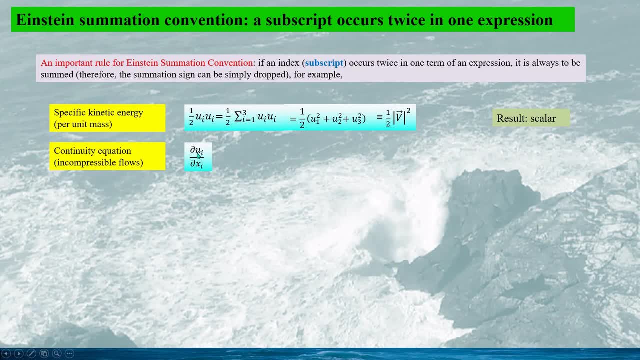 expression as this: the partial differentiation of the velocity component ui with regard to xi. In this expression the index i occurs twice. thus it means the summation as this, as this, and in a vector form it's the divergence of the velocity vector. so for the 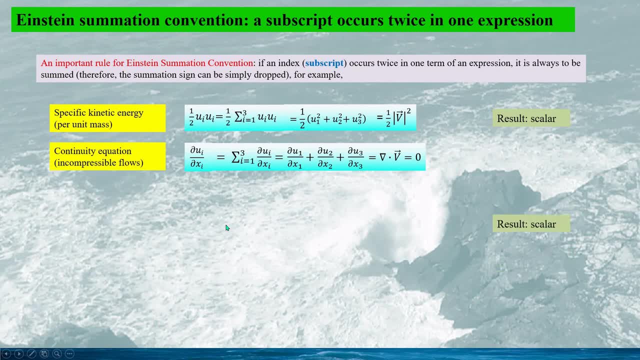 incompressible flow. it is zero. Again, the result is a scalar because the index i occurs twice. so it means the summation as this, as this, and in a vector form it's the divergence of the velocity vector. So the expression it's a scalar. so we have the continuity equation, simply. 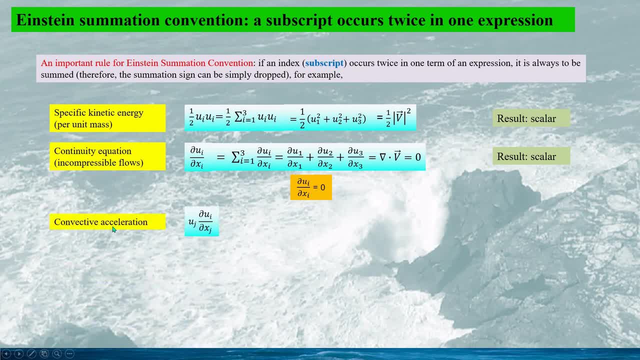 expressed as this: For the convective acceleration. the Einstein's summation expression is this: In this expression we have two different indices, i and j, and the index j occurs twice, which means summation for j from 1 to 3, so detailed expression is this and we can write this: 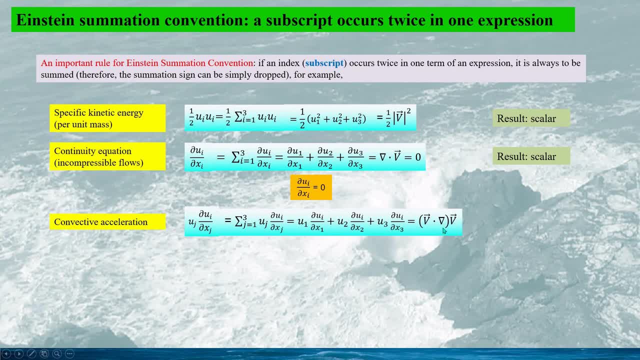 in the vector form as this. this is the convective acceleration we can see in many textbooks. The result for this expression is a vector. When we examine the type of the expression, whether it is a scalar vector or tensor, the repeat subscripts are not applicable, so in this expression, only I is the remaining. 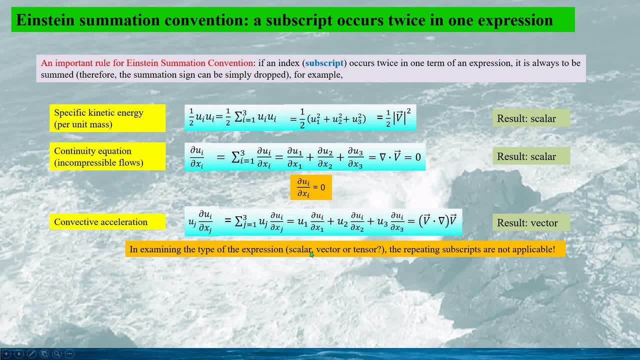 index. therefore this expression is a vector. so here is the expression: the tensor-doubled inner product. So in this case this is the one-dimensional vector. So here is the expression: the tensor-doubled inner product given by this Sij Sij. in this expression we see i and j both. 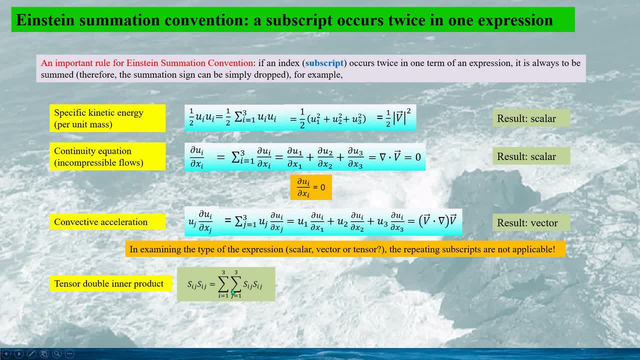 occur twice. that means the summation for both j and i. so it is given as this: if we write this expression in details, we will have this expression. so we can see the Einstein summation convention could simplify the expression very much. 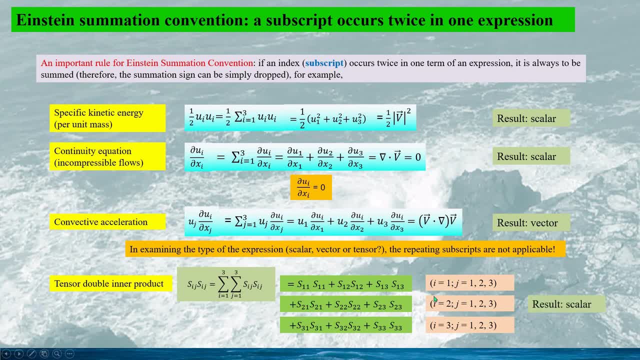 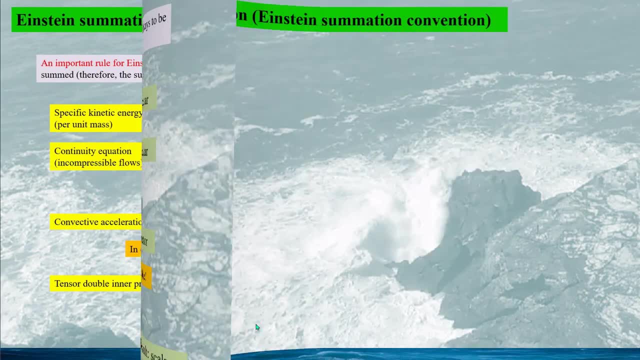 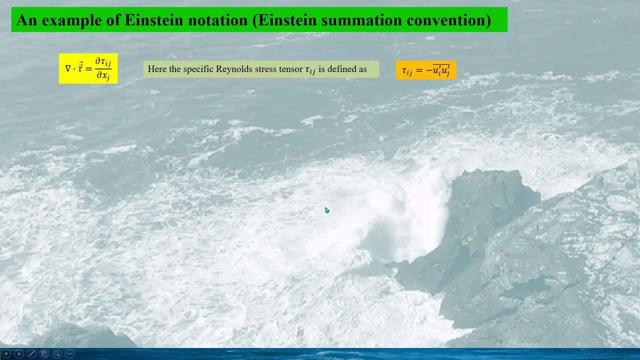 the result of this expression is a scalar, because i and j both occur twice In this slide. an example will show the Einstein notation for the divergence of the specific Reynolds stress tensor. the formula is this: the left-hand side is the tensor form for the divergence of the tensor and the right-hand side is 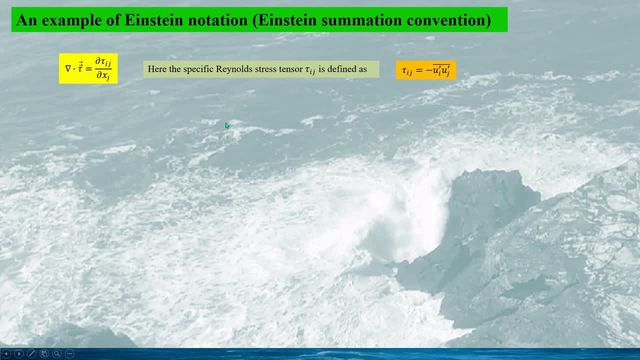 the Einstein summation convention For the direct method, the divergence of the tensor can be written as this: and if we use the definition of the Reynolds stress tensor, we have the formula as this: So write it in details. it would be something like this, and we can calculate. 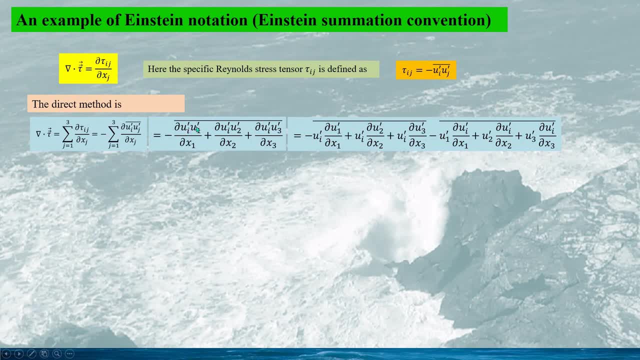 the derivations of the specific Reynolds stress tensor. so we have the expression as this: take this ui' out. we have the expression as this: if we use the conventional summation, we have the expression as this: and we can do these derivations within the summation Sigma. 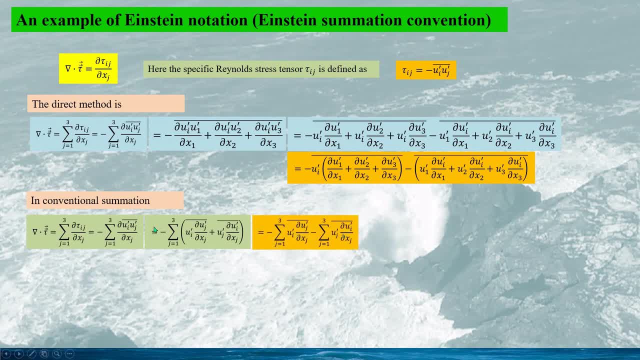 so we have this and we can write these terms as this. So you, if we compare these two, we can see the first term here and the first term. this are same and the second term are same. If we write this in Einstein notation like: 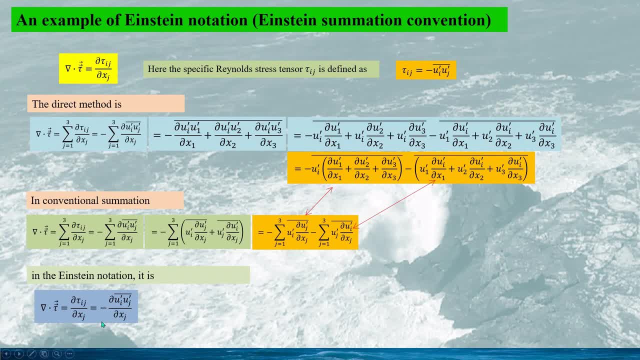 this by dropping the summation sign. so we have this and this derivation of this Reynolds stress tensor component, we have this and this and we can compare these terms. in the cycles for the incompressible flows, all these terms are zero, so these two terms would have an expression as this: and in the 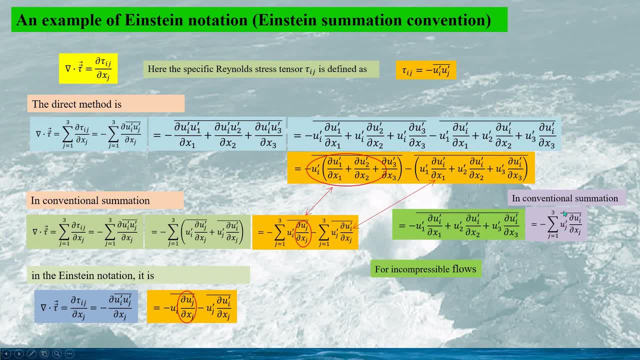 conventional summation. it has an expression as this, and here we have the term as this. this is actually the Einstein notation of this term, so we can see all these methods give the same result, but in Einstein notation the expression is the simplest. 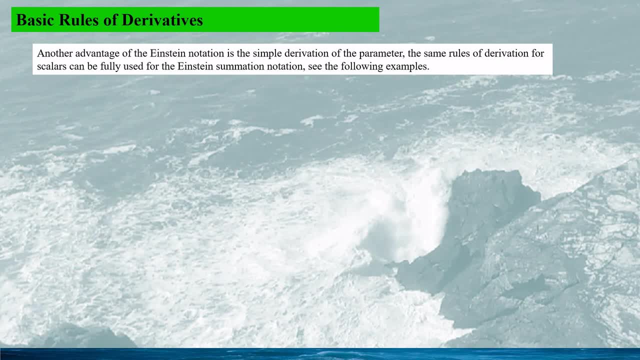 The basic rule for the Einstein notation is that the vector and the tensor can be expressed as a vector, and the vector and the tensor can be expressed as a vector in a simple form as those scalars. thus the different manipulations of the scalar, vector and tensor can be carried out like a scalar, For instance the 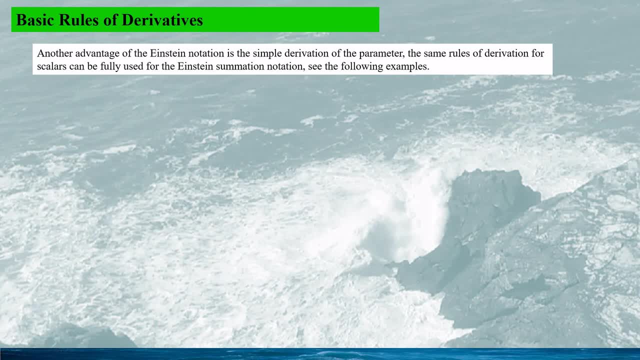 index parameter will keep the same type. if the derivation is with regard to a scalar, for instance time, so the density of the vector and the tensor will be the same type. if the derivation is with regard to a scalar, for instance time, so the density. 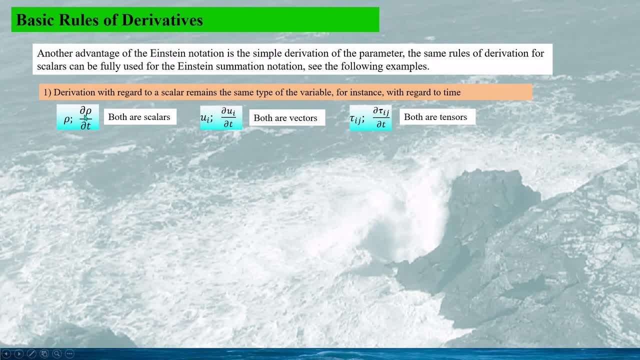 know a scalar. its derivation with regard to time is the scalar and the velocity ui the vector. its derivation with regard to time t is the vector 2, and tau ij is the tensor. its derivation with regard to time is the tensor, However more complicated. 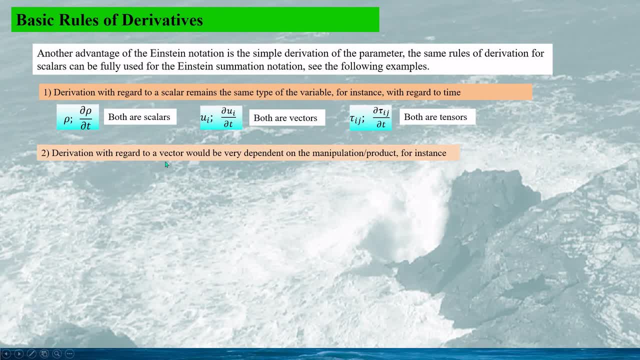 situation would be the derivation with regard to a vector which would be very dependent on the manipulations and the products, For instance the density a scalar. its derivation with regard to a vector: xi is a vector given as this zenerbler density Rho. 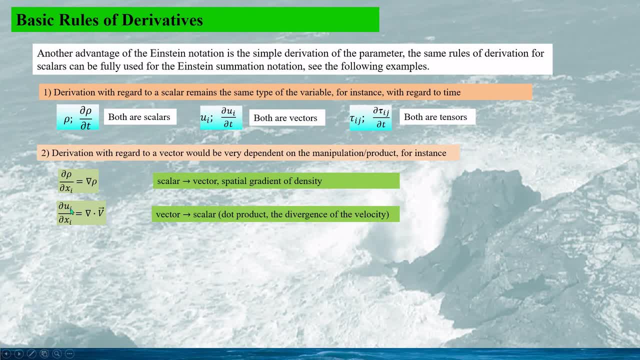 The derivation of the velocity ui with regard to a vector xi. it is the inner product of a lambda and the velocity vector. so this result is the scalar. and if we look at the derivation of uj with vector xk, consider the Levy-Helmholtz. 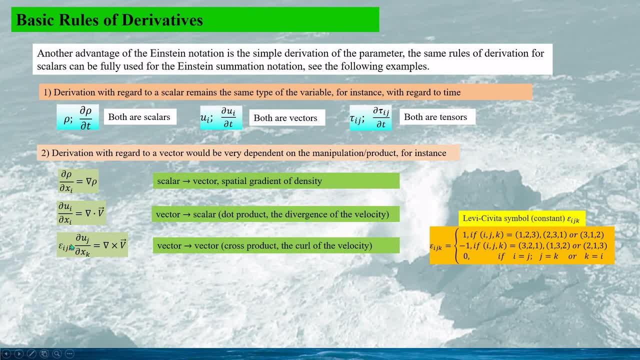 ratio, zeta symbols, EPSILON, ijk. so this expression is the core of the velocity. Levy-Helmholtz became the velocity vector. so the result is a vector, The velocity vector ui, its derivation with regard to a vector xj. 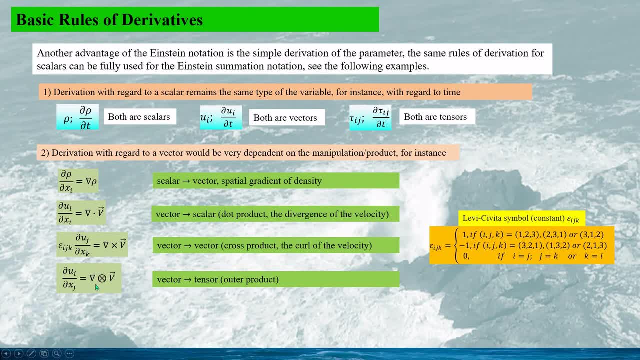 would be the velocity vector ui, a tensor given as this Labrador out-timing a velocity vector, and the tensor TAU ij. its derivation with regard to a vector xj equals to the divergence of the tensor, that is, labrador dot times the tensor. 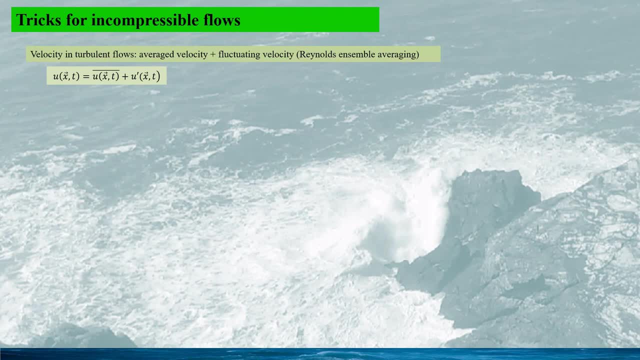 In this slide we will look at some tricks for the incompressible flows. For turbulent flows, the velocity can be written as the main velocity vector plus the fluctuating velocity, or simply expressed as this form here: U is the averaged velocity, u' is the fluctuating velocity. 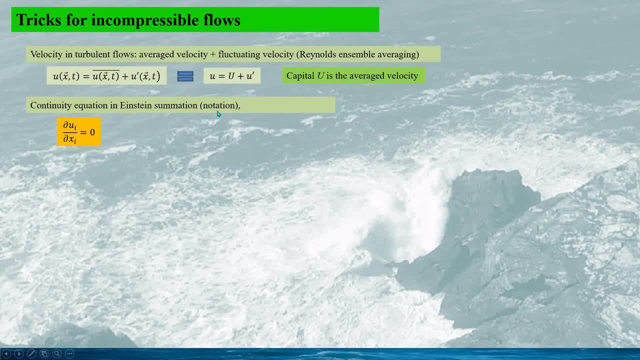 the continuity equation in Einstein's summation notation is given as this. so we substitute the expression of this into the continuity equation. we have the expression as this. so from this equation we can obtain the relation as this for the averaged velocity, capital U and the fluctuating velocity, and we can see: 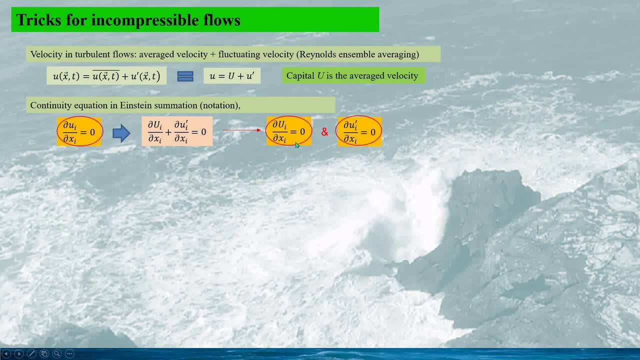 the continuity equation for the velocity, for the averaged velocity U. this equation is given as this and the fluctuating velocity are all same. Now we can have a look at the tricks. we use the Einstein summation. the first one is the expression this: so use the rule of the calculus. we can have the 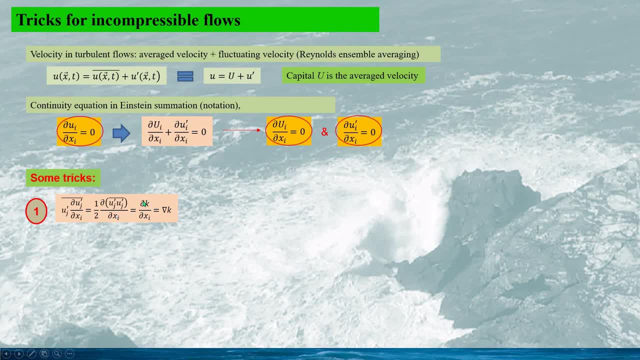 expression this and use the definition for the turbulent kinetic energy and this is the gradient of the turbulent kinetic energy and we look at these two terms and again use the rule of calculus- we have the expression as this- and substitute the Reynolds stress tensor TAU ij we. 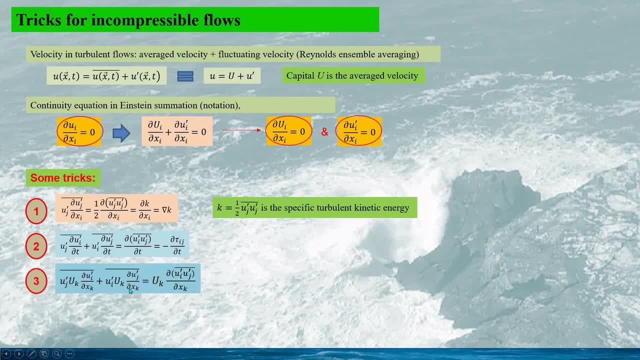 have the expression as this. The third expression is as this: the two terms and we can apply the rule of the calculus. we have the expression as this Here: capital UK is a constant with regard to the averaging operation, so we have this expression. 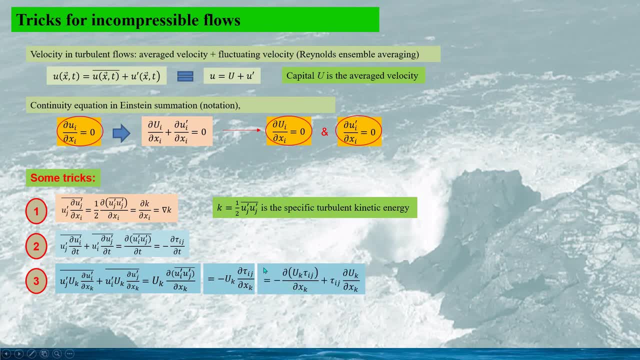 so we can make a further derivation for this expression. we have this and the. if we apply the continuity equation for the incompressible flow, this term would be zero. thus we have the final expression as this. The fourth expression is given as this, so we can use the same rule: get the.